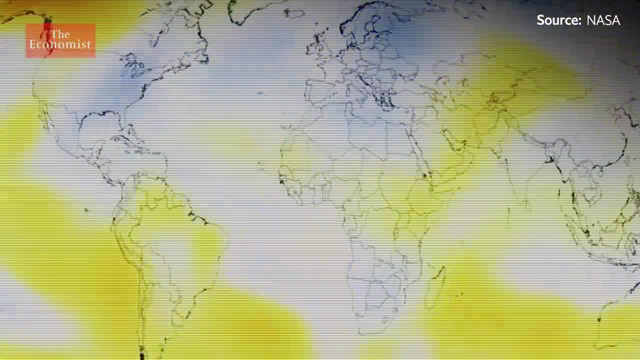 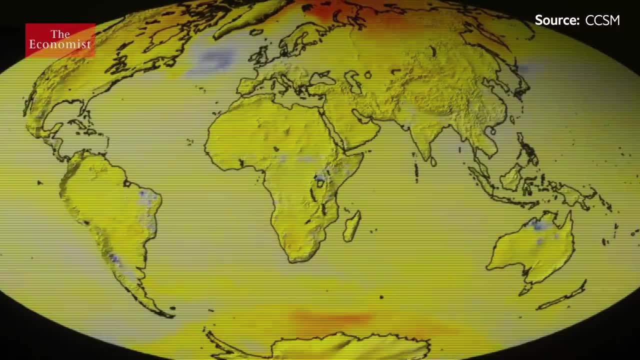 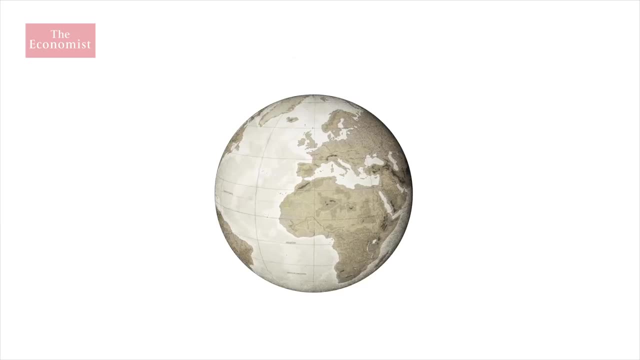 That was one of the first ways that climate models began to illustrate the fact that greenhouse warming really was likely to be a problem in the 21st century. For all their complexity, these models have limitations. Although you're cutting the atmosphere into millions of cells, the atmosphere is a very big thing. 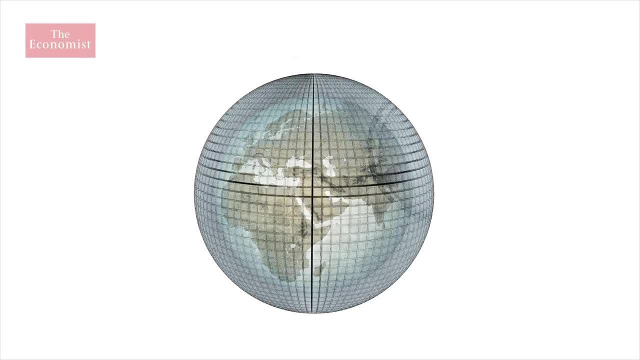 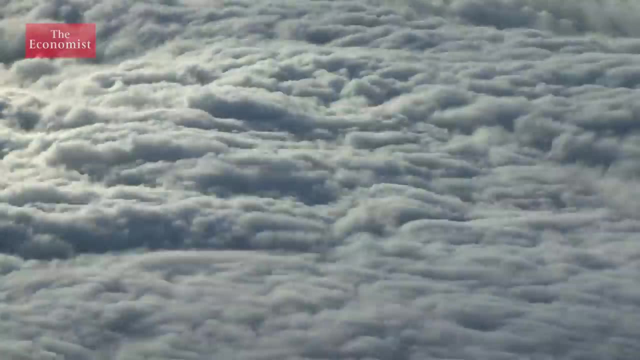 And a millionth of a big thing is still a pretty big thing. So the cells tend to be maybe hundreds of kilometres on a side. This means the models often struggle to capture details like cloud cover, and clouds play a key role in climate. 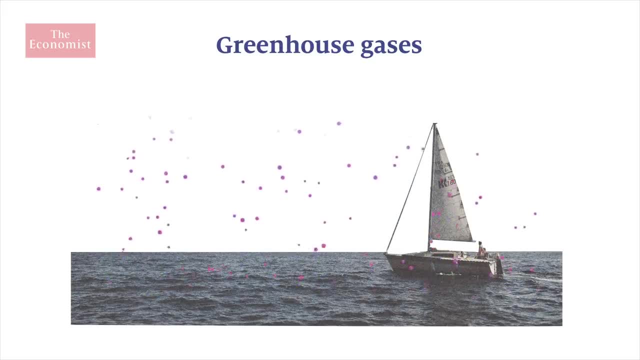 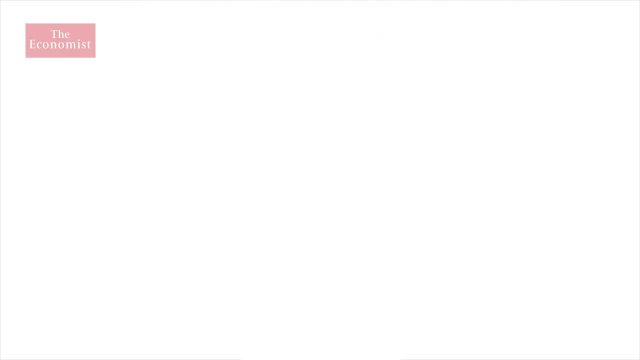 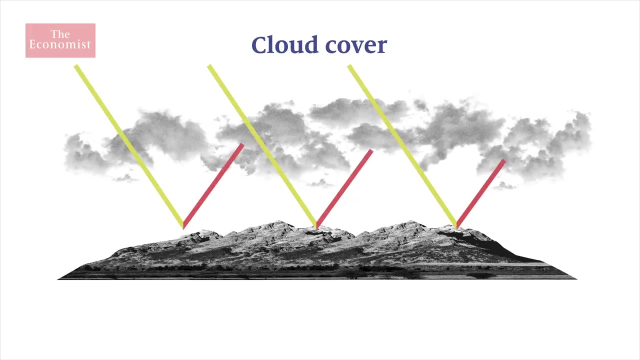 As greenhouse gases make the atmosphere warmer, they change the amount of water vapour it can hold and how air rises and falls. That in turn changes the amount and character of cloud cover. Depending on where clouds form, they can either trap sunlight, which warms the planet. 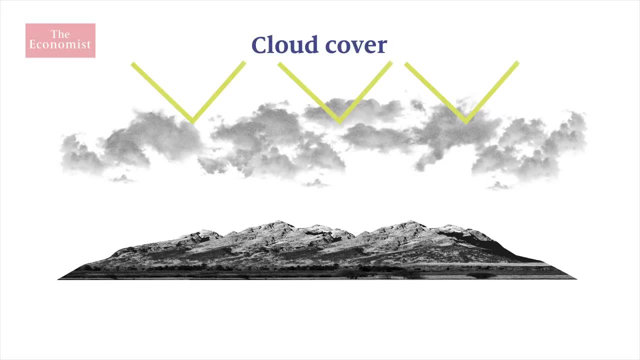 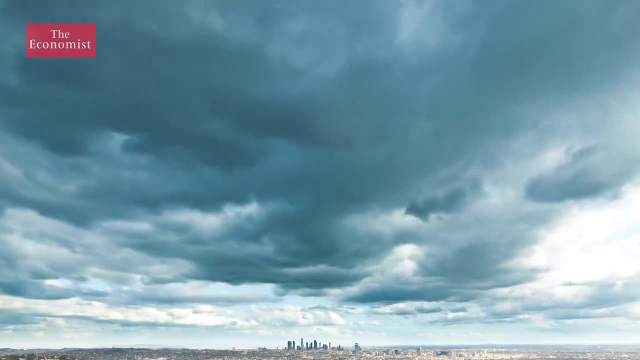 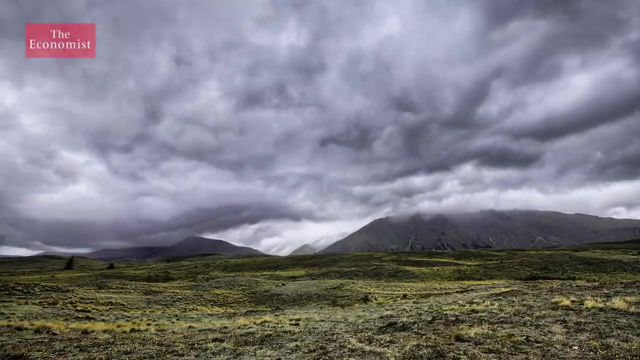 or reflect it back into space, Cooling it. And some processes which govern cloud formation work on a very small scale, So you can't actually model those precise processes in the computer models. So you have to build various different rules of thumb in. for what would you expect the clouds to be doing? 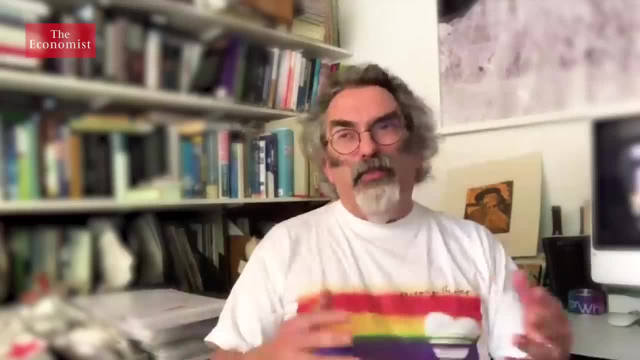 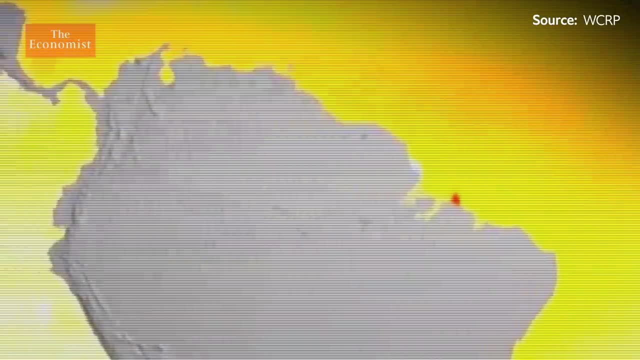 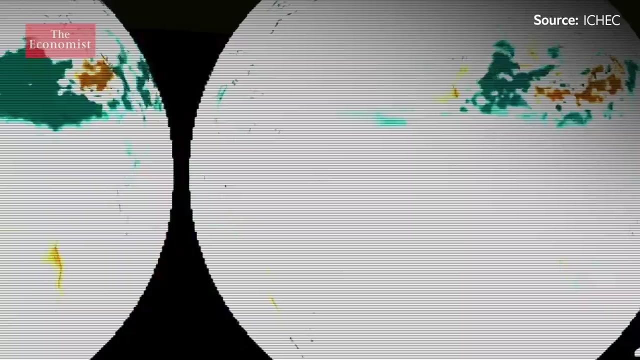 How you do. that means that your model will behave differently compared to someone else's model, where they do that in a different way. Dozens of these models exist, Run by teams all over the world. The modelers all want to capture the Earth as close as possible to how it is. 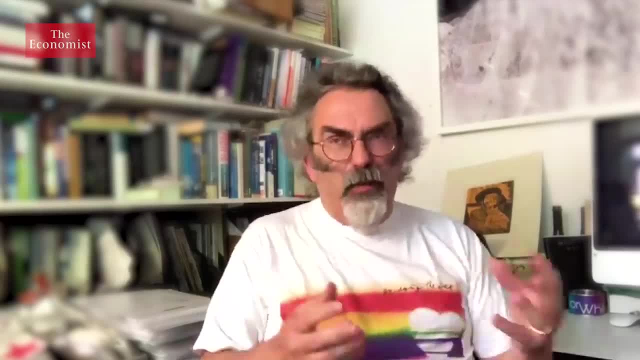 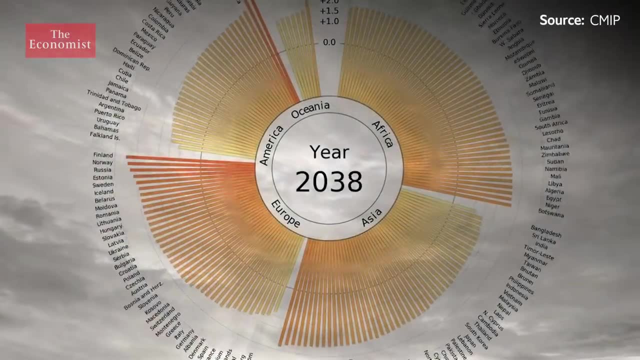 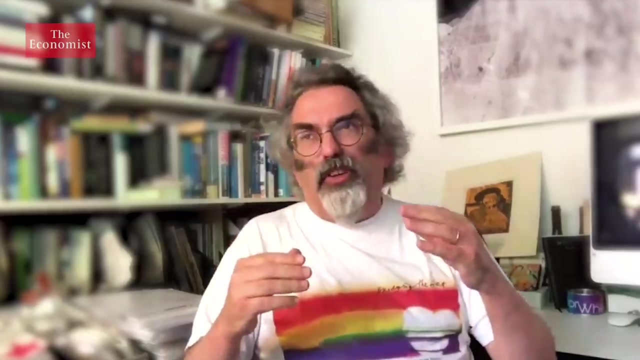 but their assumptions about how that actually works differ from model to model and the ways that they implement those assumptions change. Some models tend to people say, run hot, so they tend to provide more warming for a given amount of carbon dioxide, and some models tend to run a little cold. 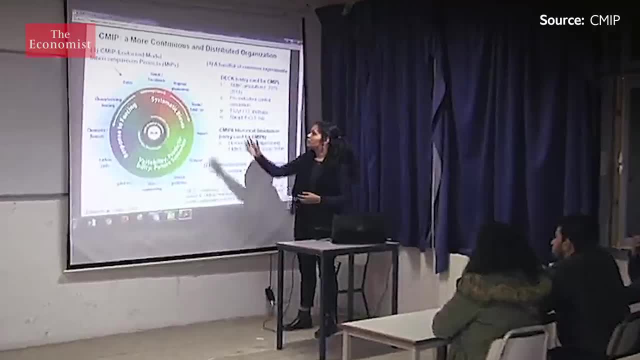 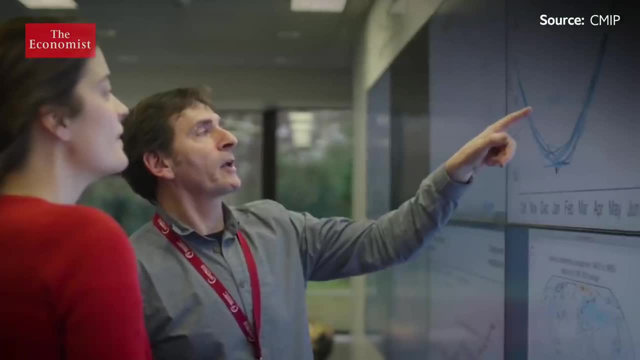 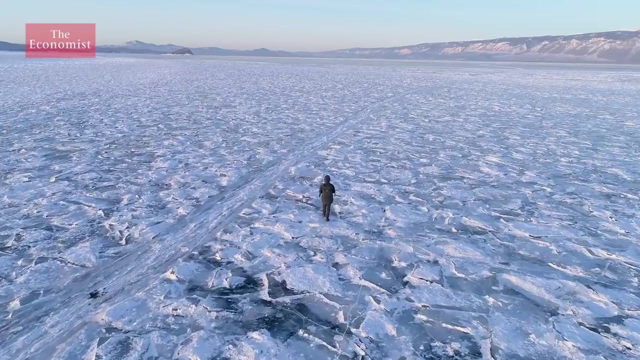 Every few years the models are brought together, fed standardized questions and then their results are compared. This helps scientists understand the strengths and weaknesses of different climate models and improves them. Of course, it's impossible to assess the models' future projections. 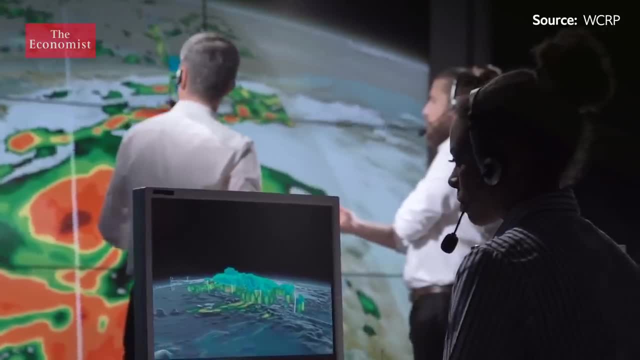 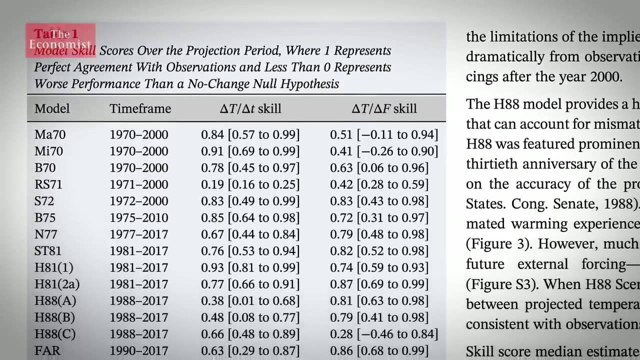 but what researchers can do is compare the success of models from previous decades. A recent report compared the models from the 1930s to the 1970s to the 2000s, And it found that by and large they were reasonably good. 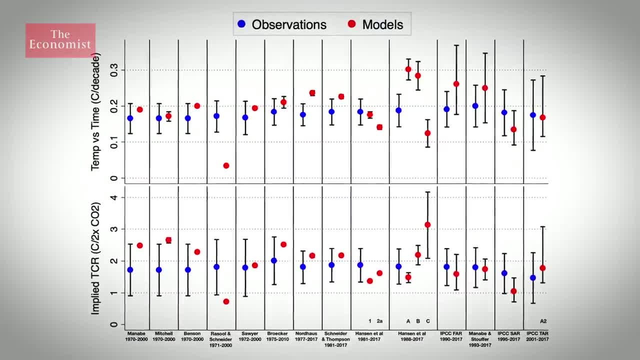 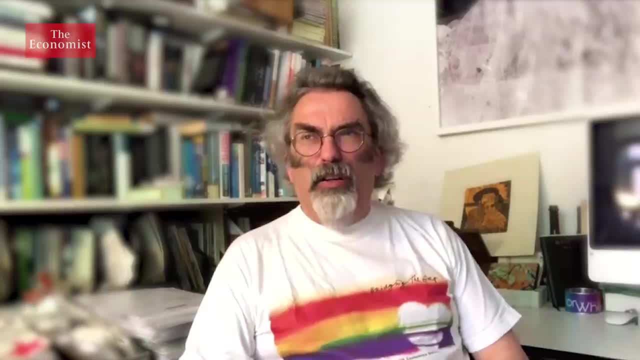 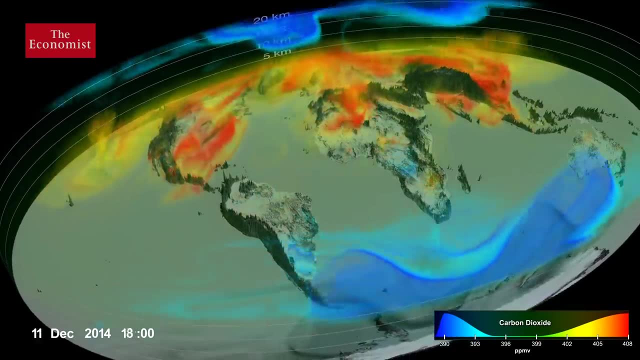 The warming that we'd actually seen sat within the error bars for most of them, So it gave us a general sense that these things weren't completely out of the park. The climate models are getting increasingly complicated, capturing more aspects of the Earth, But there is one element that is impossible to model. 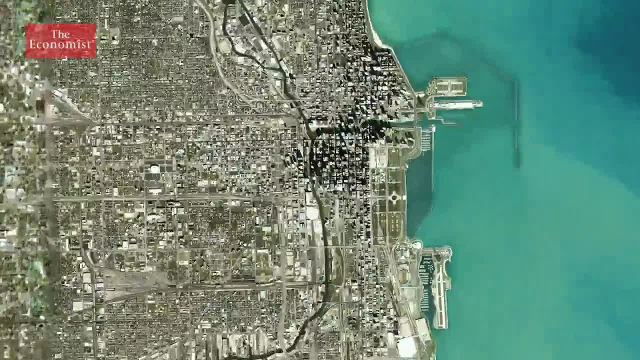 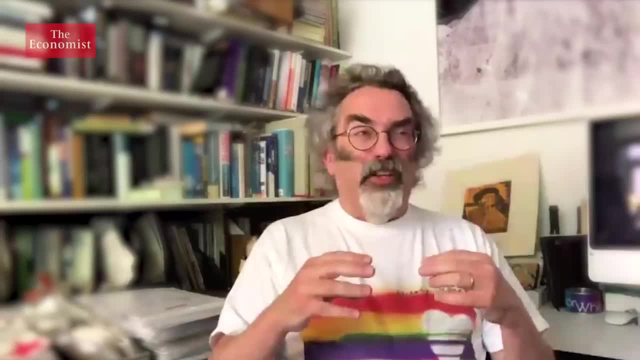 and it is the biggest contributor to climate change. The thing about human activity is that you can't get it inside the model. The model deals with sort of like physical laws of chemistry and physics and biology, So there's no way the model can say: 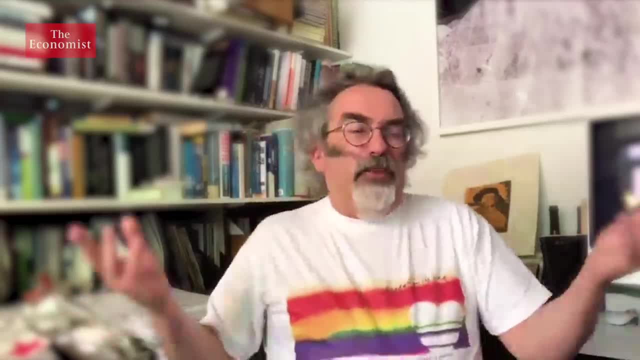 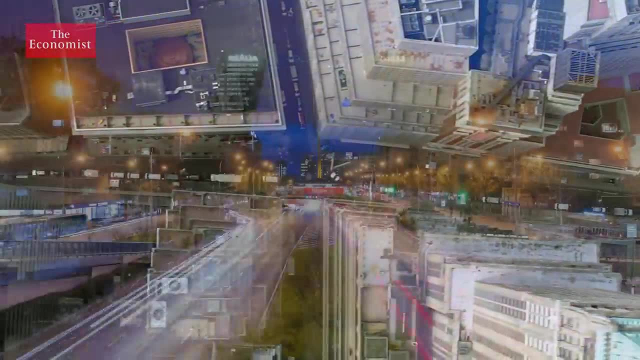 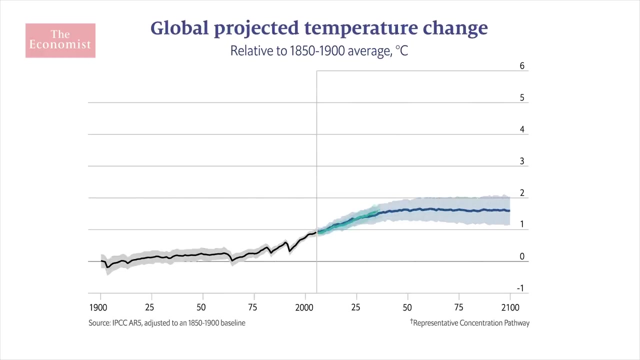 well. in 2050, America will have stopped emitting carbon dioxide. Instead, scientists take simplified results from these climate models and run them through economic models. In 2013,, scientists used these models to examine the effect of different climate policies on the future temperature of the planet. 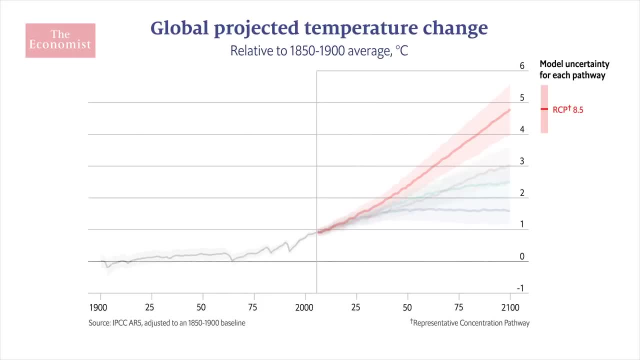 The first looked at what would happen if there was continued large-scale use of coal. The second if there was continued use of fossil fuels but some use of renewable energy. The third if there was a much higher uptake of renewable energy. And the fourth if there was a lot of use of carbon capture technology. 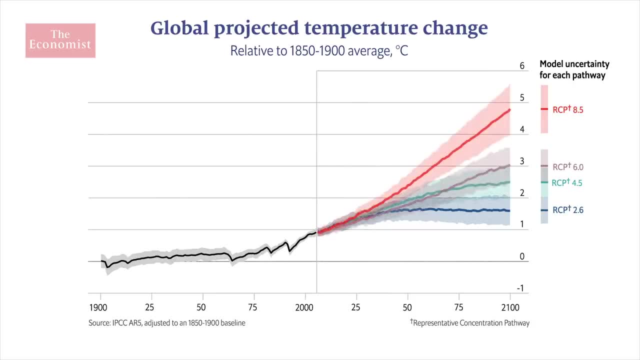 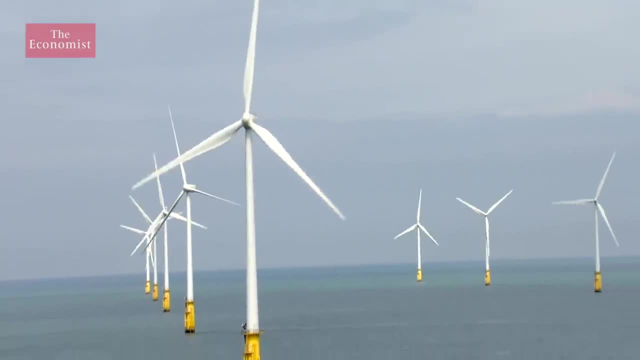 and more land to grow biofuels. The striking thing about those comparisons- and by other comparisons that will come out later- is that only really tough climate policies get you the sort of trajectories which keep the temperature, in the words of the Paris Agreement. 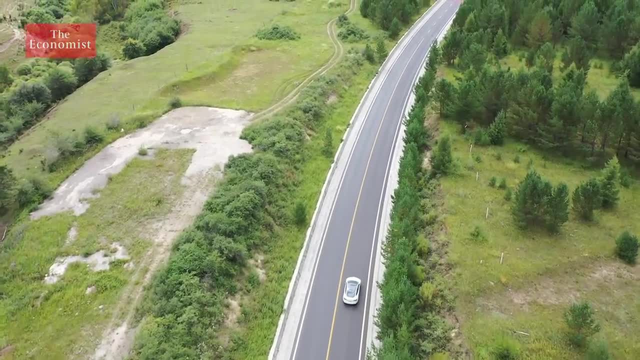 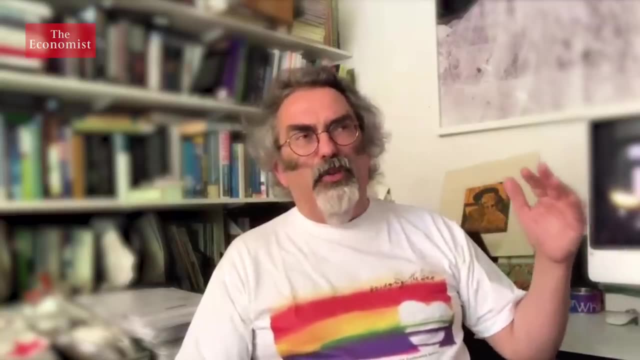 well under two degrees above the pre-industrial. What these models tell us is that the current level of emissions reduction is not remotely enough to have any assurance that you'll stay under two degrees, even less sort of like close to 1.5 degrees. 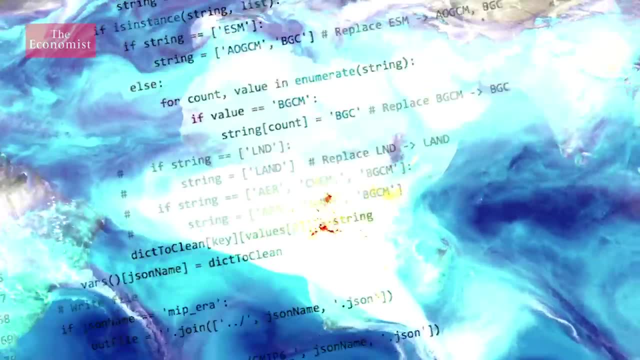 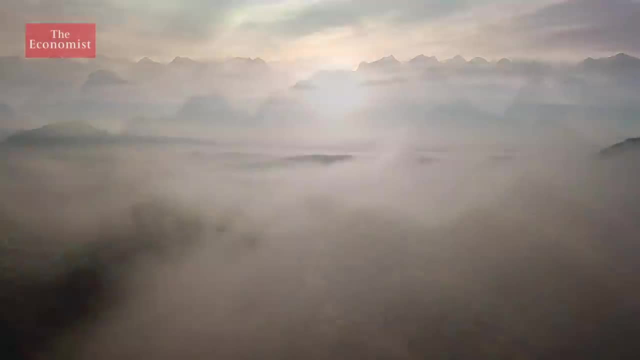 Climate models don't predict the future and they're not perfect. There is a long way to go before they fully represent all of Earth's intricate processes, But for now they are the only way that scientists have of understanding how damaging an increase in carbon dioxide 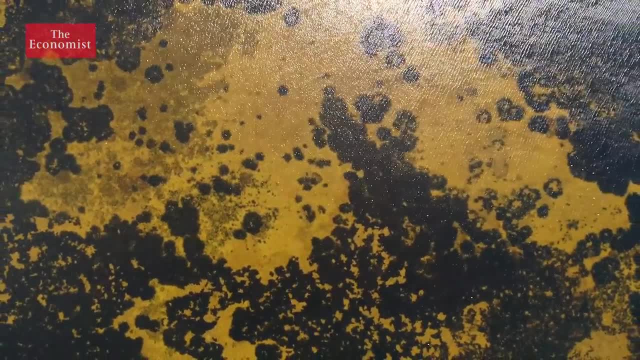 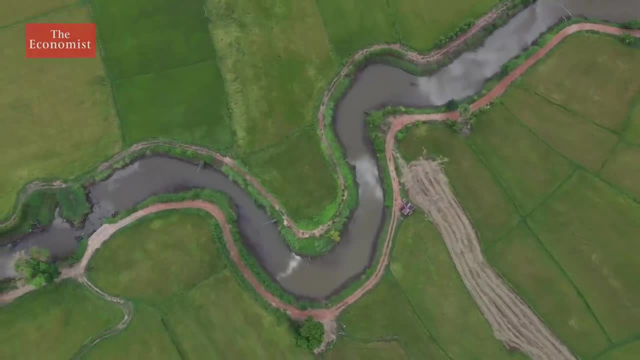 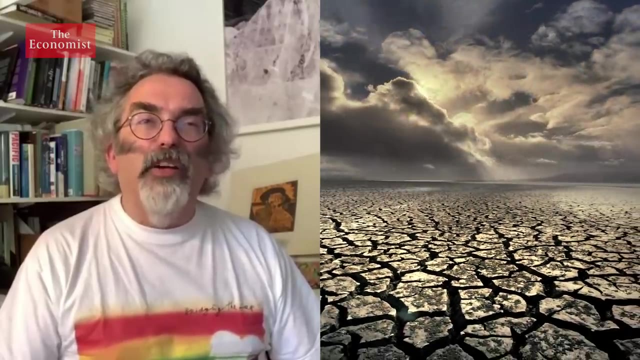 will be for the planet. Ultimately, the solution to climate change won't lie inside models, but rather what humans choose to do with the information they provide. I'm Oliver Morton. I'm the Briefings Editor at The Economist. We've written a series of climate briefs. 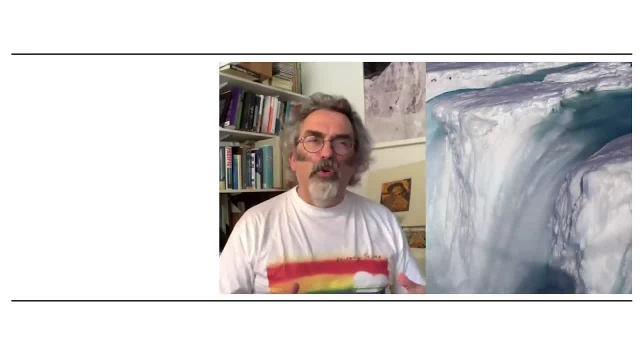 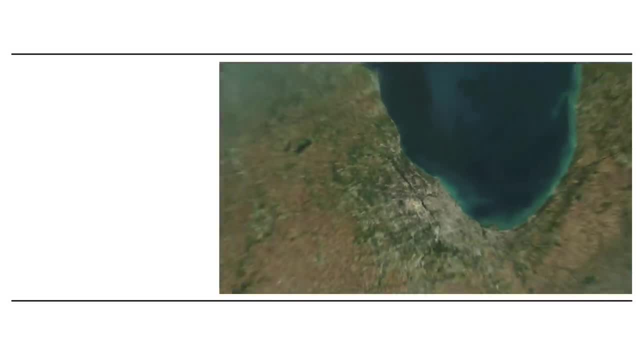 to cover the basics- and a bit more than the basics- on all sorts of aspects of the climate crisis that's facing the Earth. You can read them all at the link opposite. Thank you for watching. 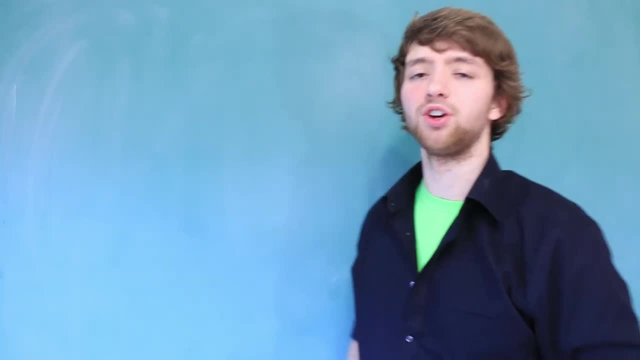 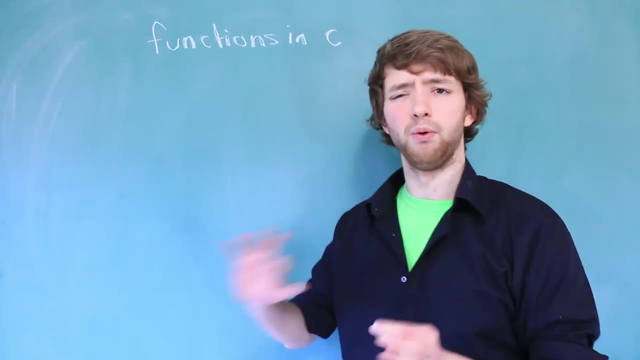 What is up, everyone, It's Caleb from Caleb the Video Maker 2.. In this video, we are going to introduce using functions in C. I've talked about this a little bit and I mentioned a little bit about what functions are and how to use them, but I wanted a video just to introduce a little bit. 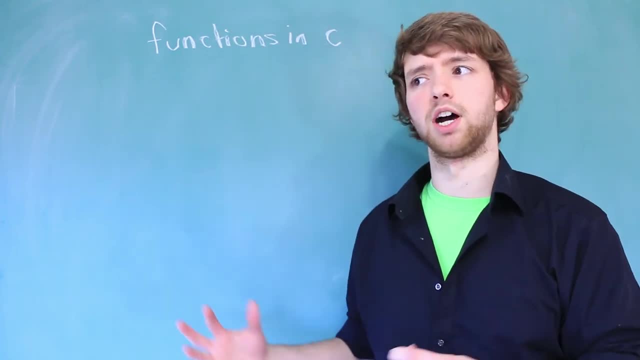 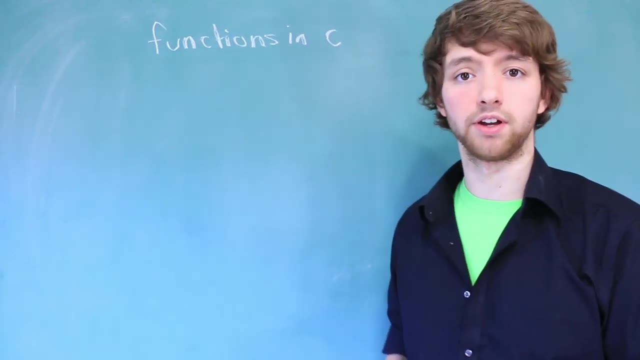 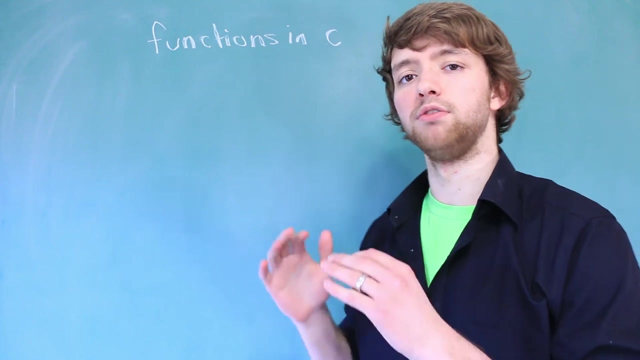 more detail. So that way, as we use functions, you're not like what the heck is he doing? So that way you have a better idea of what's going on. when we start typing out more code and everything As we move on in this series, we are going to start moving more systematically. 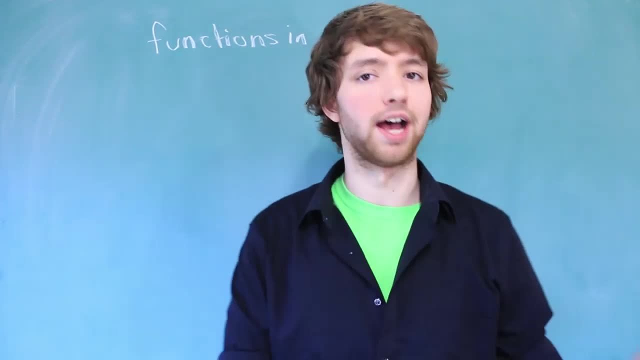 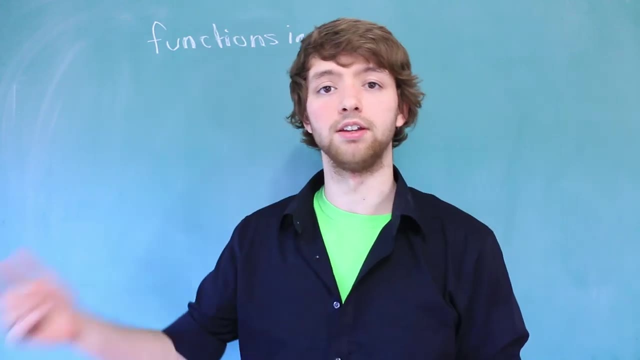 through concepts in C, rather than what we've done in the last five or six videos where we just kind of give an overview of a bunch of things. That's because we need to go in more detail in order to understand everything we need to know Specifically farther in the future. 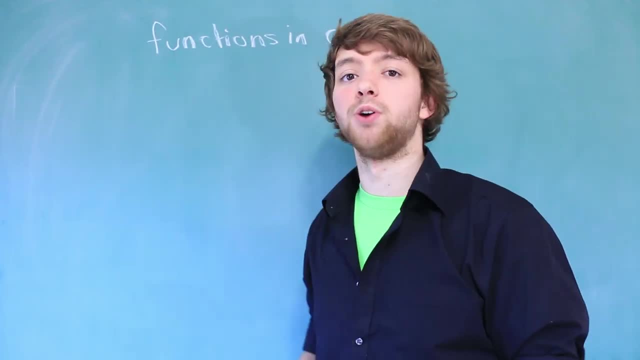 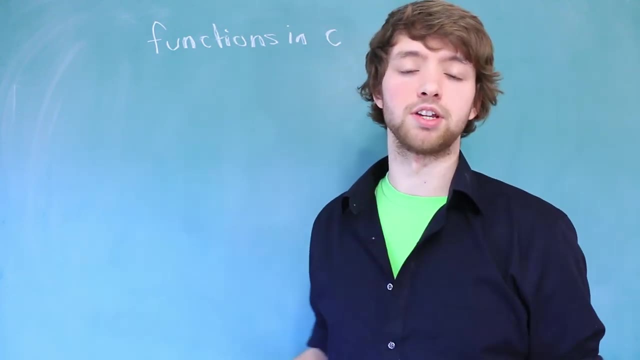 we are going to talk about functions in depth, So don't feel like you have to know everything from this video. And if I've already told you basically everything already that I talked about in this video, that's okay. I just want to centralize it in one. 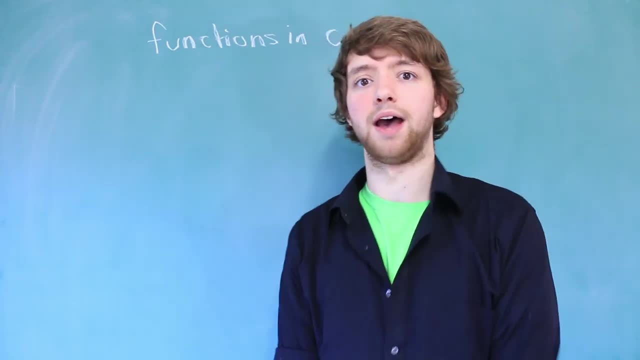 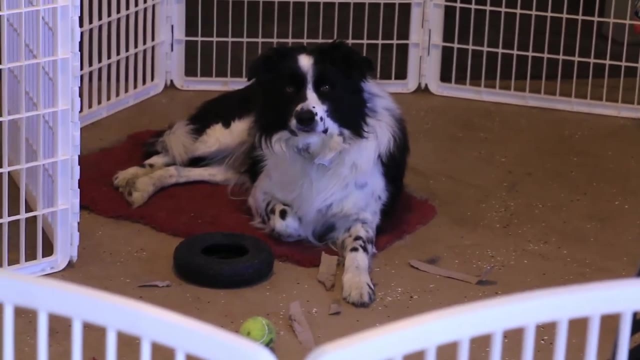 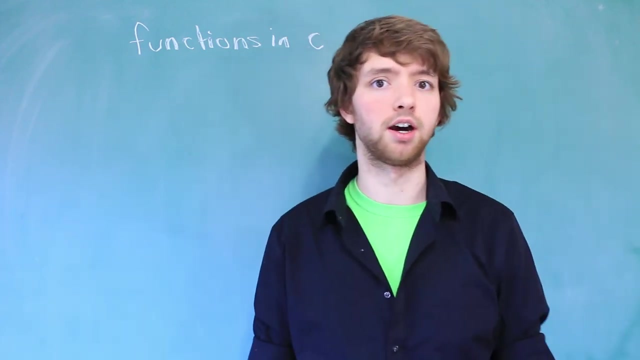 video so you can have it for your use. So, with that being said, let's begin. What is a function? A function can be used to call or execute multiple statements at one time. Now, the computer actually does go through each statement one at a time. 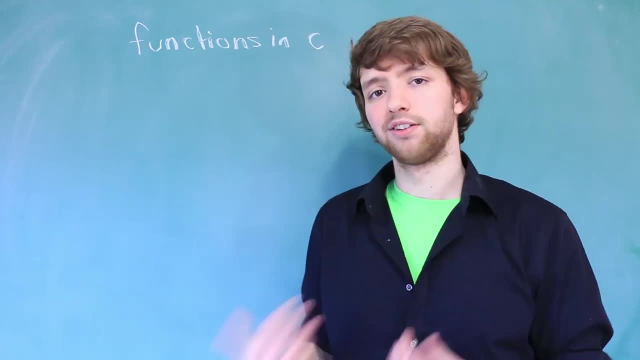 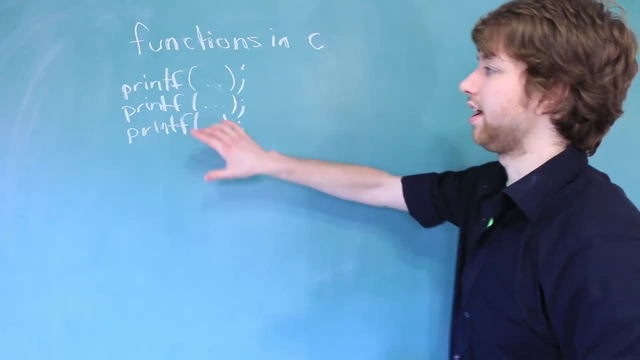 But for us as programmers, we only have to say one thing. So, for example, if we are trying to print three things to the console, our code might look something like this: Now, technically you wouldn't have to have three printf statements.